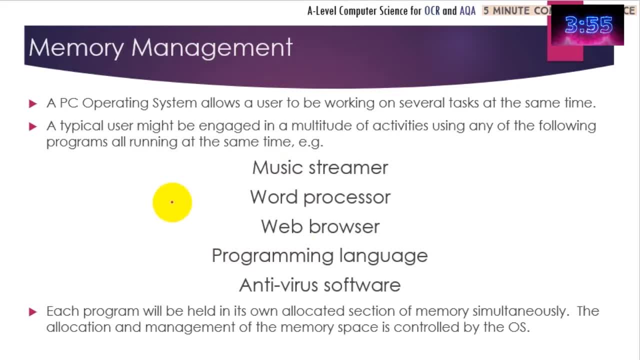 different programs can be running at the same time, But to you and me, the users, it appears that our operating system is multitasking, So memory management is absolutely key here. You might well be running a number of different programs, like a word processor, a web browser. 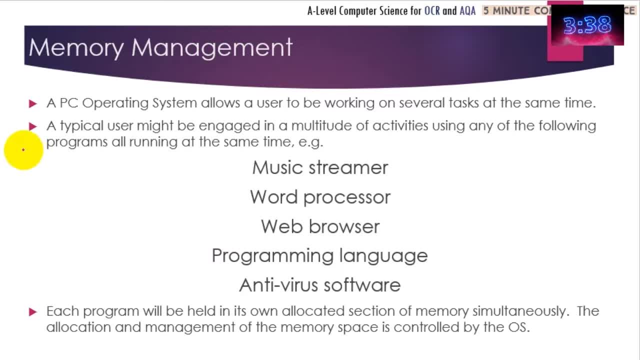 you might be doing your computer science homework or whatever it is, But of course the CPU can only process one instruction at a time. But by managing memory you can run a number of different programs at a time. By managing memory, managing the RAM, managing the hard, 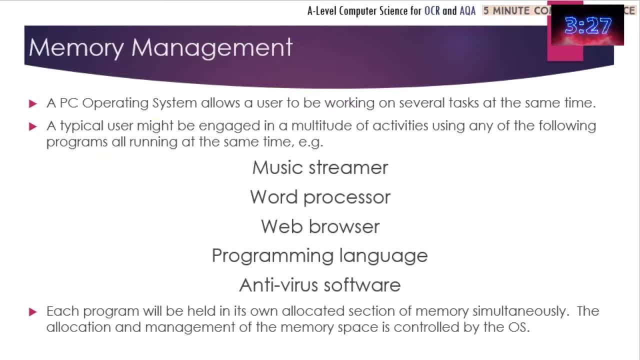 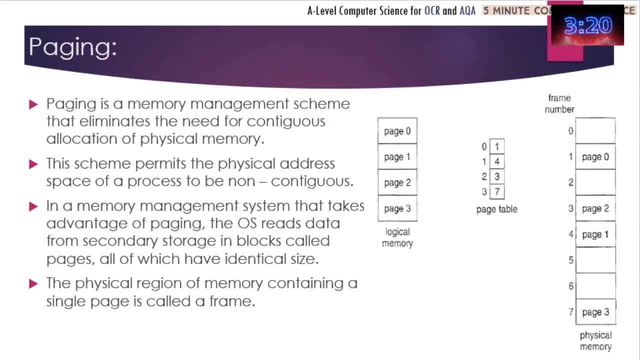 drive, etc. It can appear as though you're multitasking, and that's part of the job of the operating system. It's controlling the CPU. Here's a little technique that you need to be familiar with. It's called paging. Now, in an ideal world, when we save instructions, 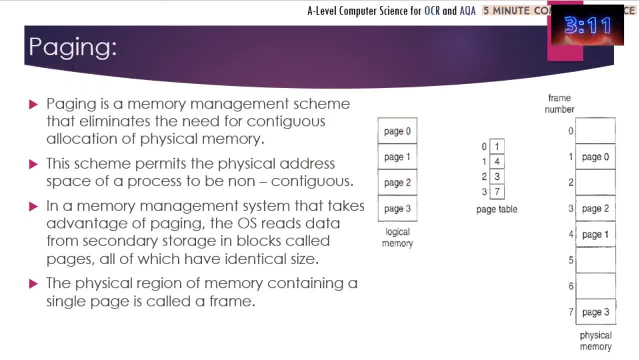 and data into RAM. we want everything to be physically next to each other, And that'd be helpful if the first line of couple of lines of code were on page zero and the next line of code were on page one, etc. It'll be lots of different parts or, in this instance, frames, So this is the order we 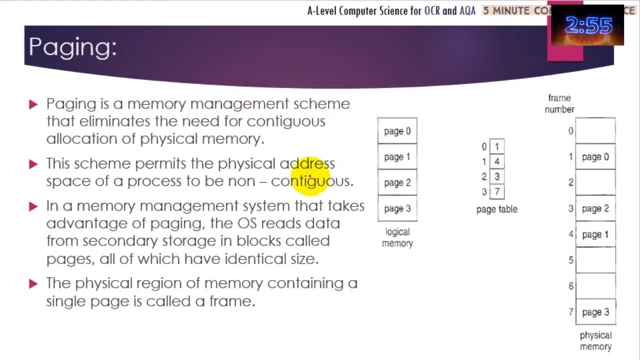 want to access it: Page zero, then page one, page two and page three. But what the operating system does? it keeps a paging table to keep track of where everything is physically. So page zero is actually in frame one. page one is in frame four. page two is in frame three. 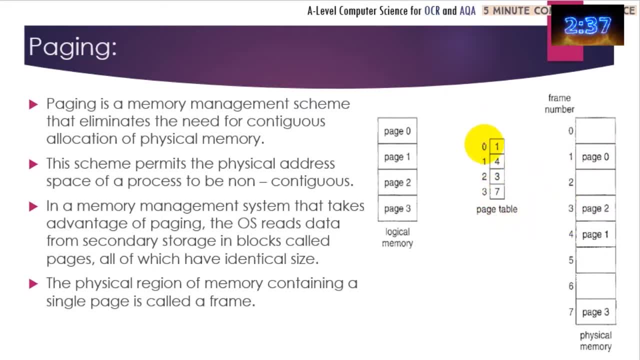 and the page table knows this. So the page table knows that in order to access frame zero, we need to go There. Okay, And in order to access the next set of code, whatever it might be, page zero, we need to go to frame four. And then, in order to access the next frame, page two- we need 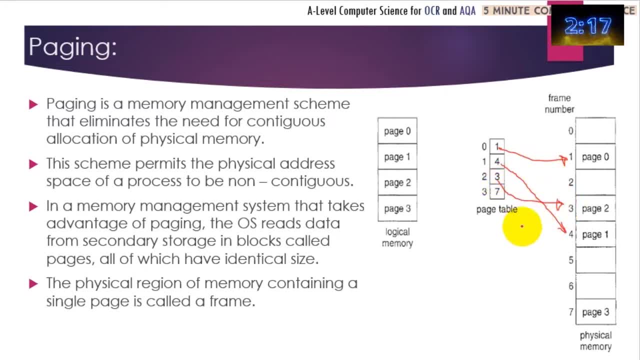 to go to frame three, And, of course, RAM is just filled up as and when it's required, And so a page table is used to ensure that all the different parts of the program that are needed can be accessed whenever needed. Here's another example of what you need to. 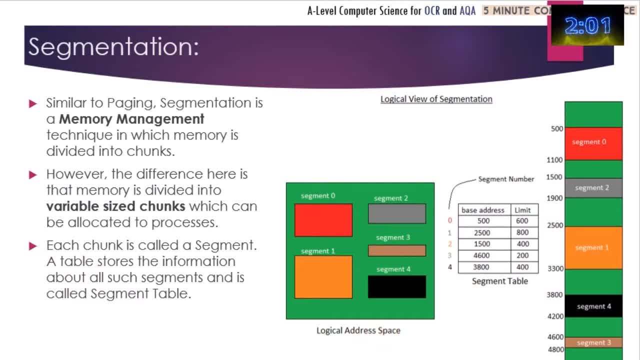 be aware of. So on a page three, page four and page five, you need to sign up in the PDF. The pre-сяid y's are required so that, in particular, they can go back to steak file F and then they.